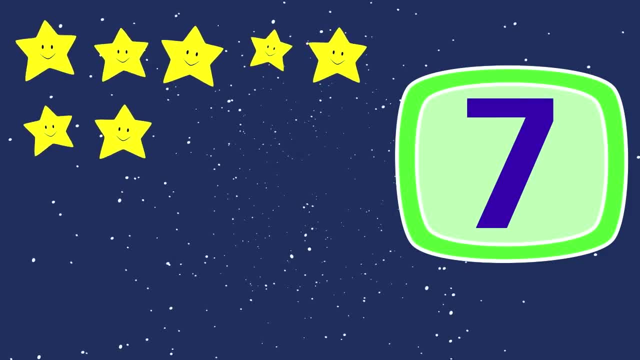 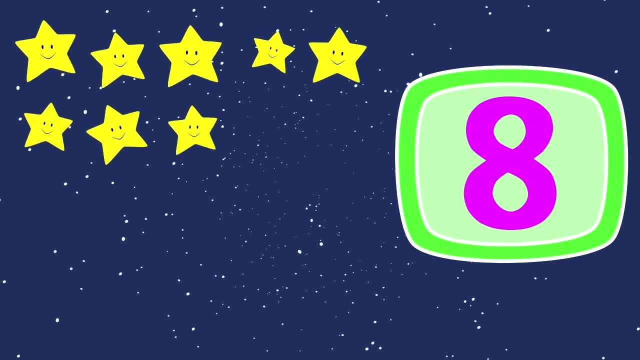 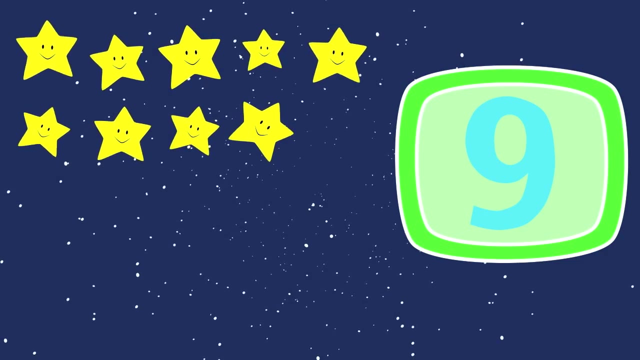 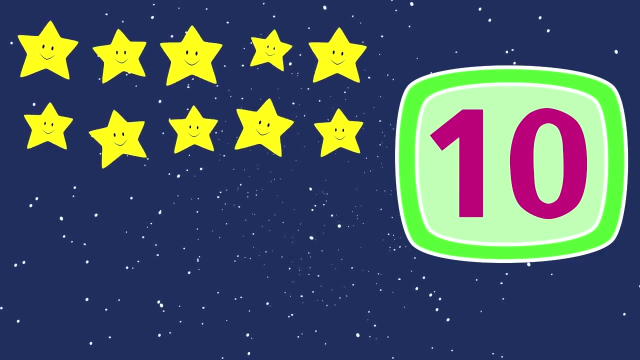 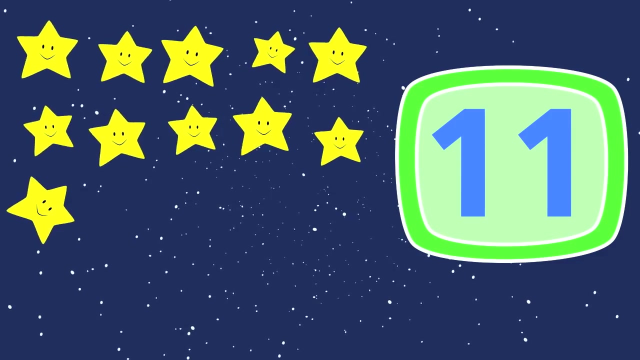 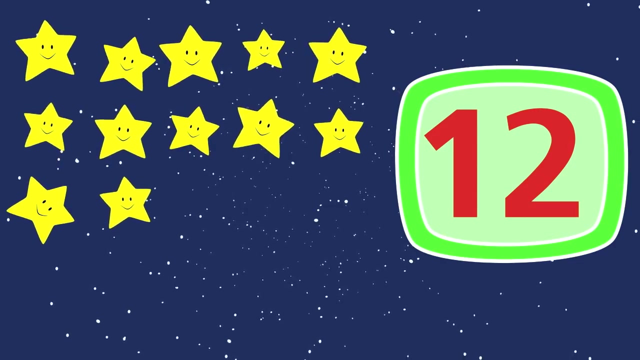 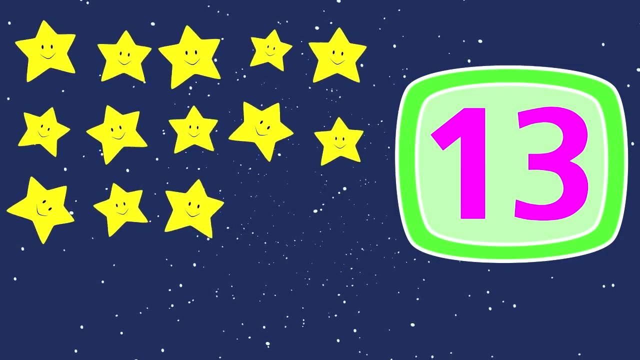 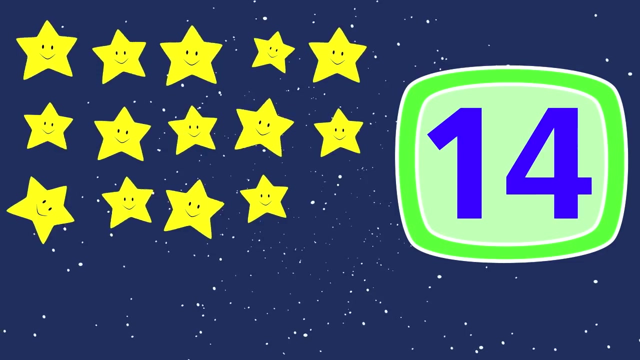 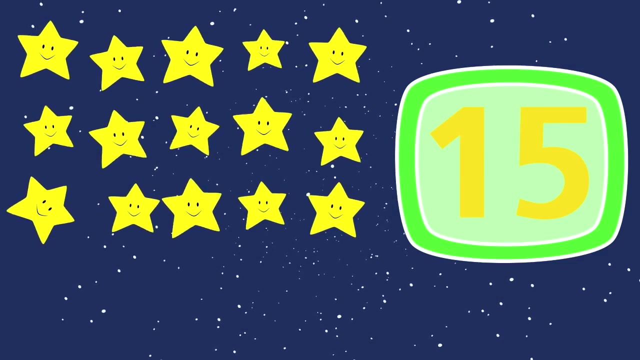 7,, 7,, 8,, 8,, 9,, 9,, 10, 10, 11, 11, 12,, 12, 13, 13, 14, 14, 15,, 15, 16,, 16. 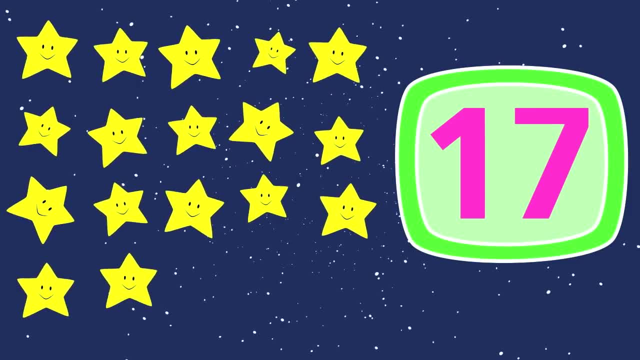 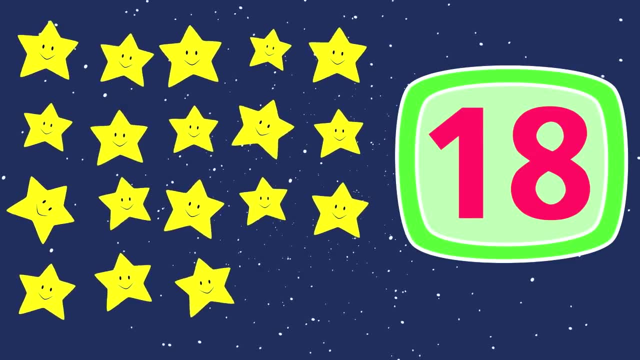 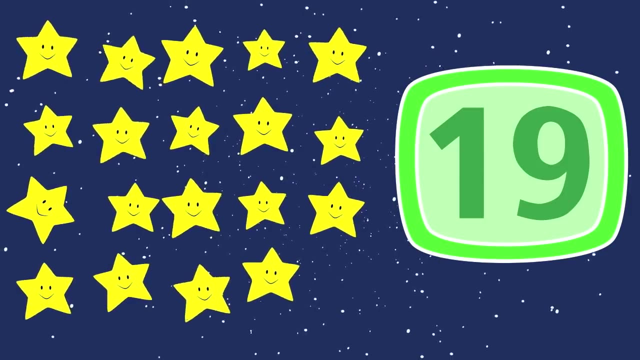 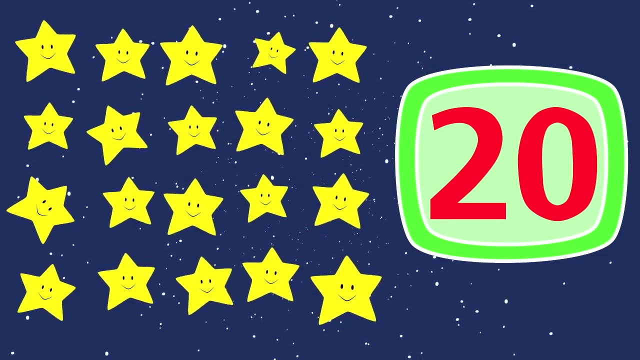 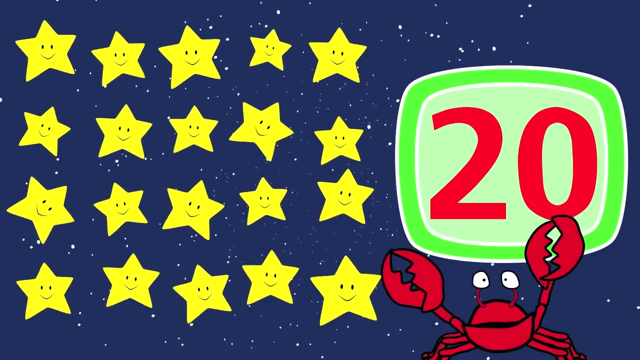 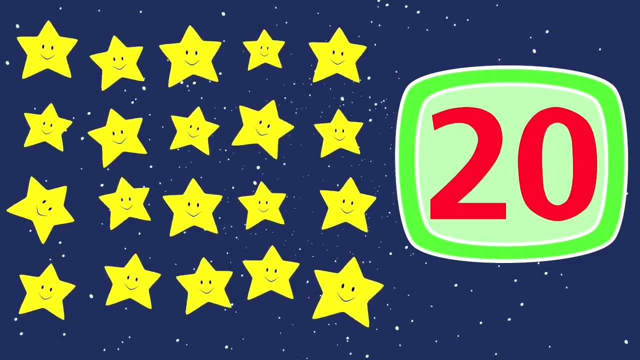 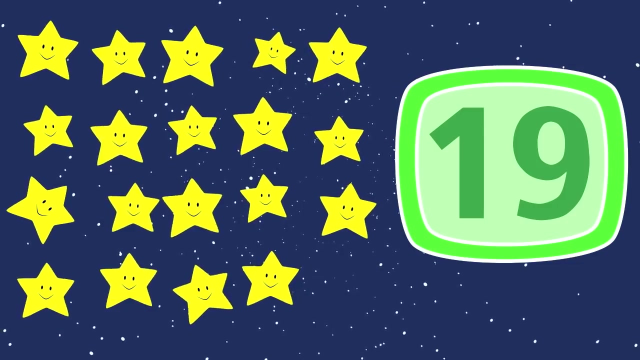 17,, 17, 18,, 18, 19,, 19, 20,, 20, 20 Outstanding. Now let's count backwards from 20 to 1.. 20,, 20, 19,, 19, 18,, 18. 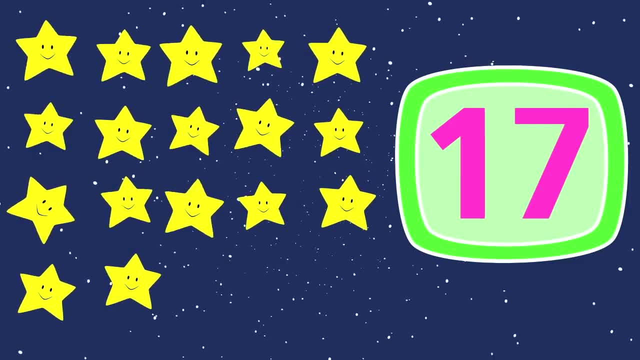 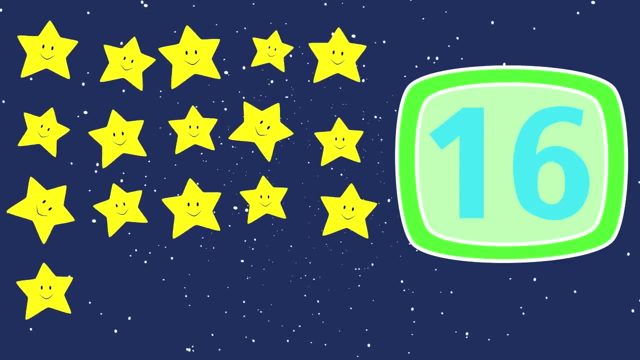 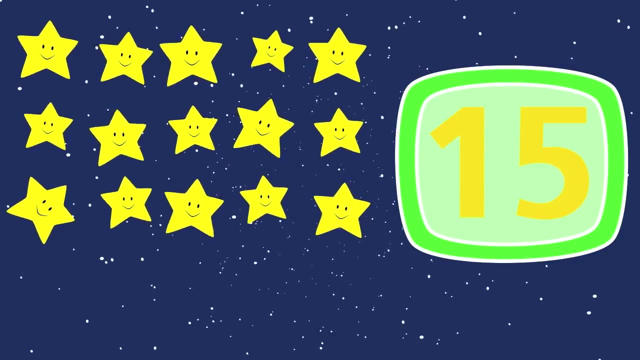 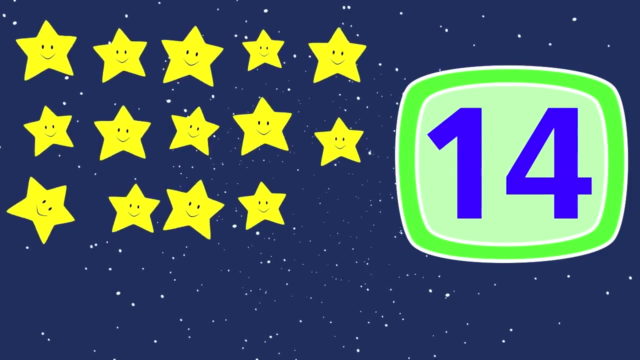 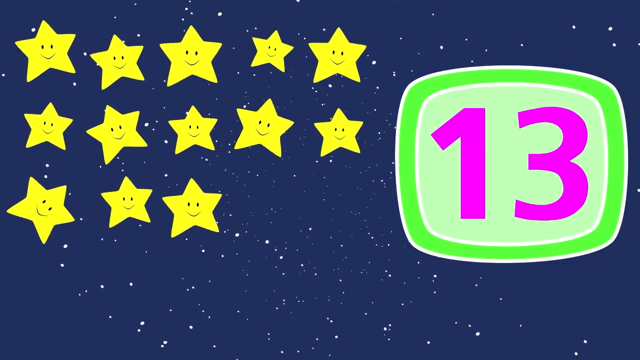 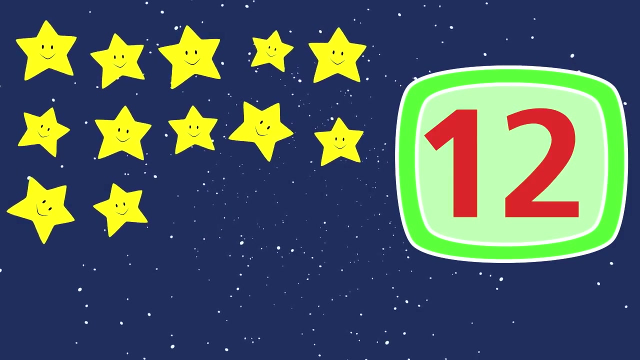 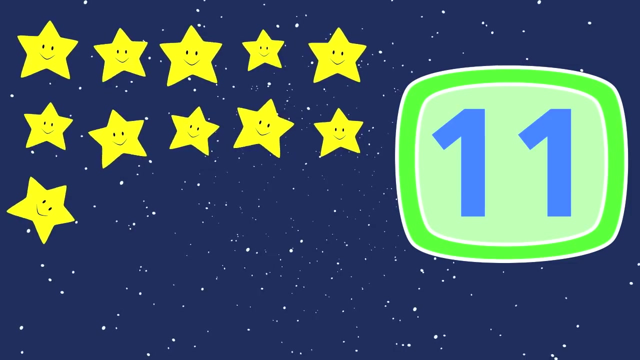 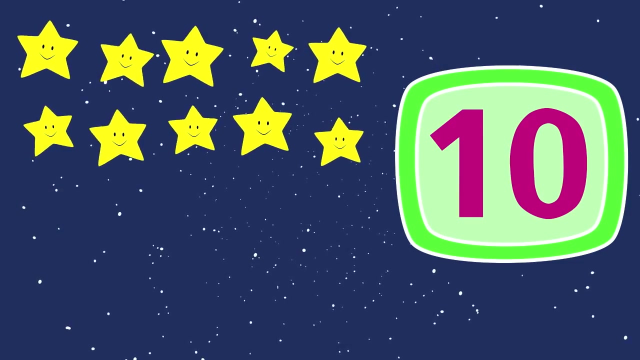 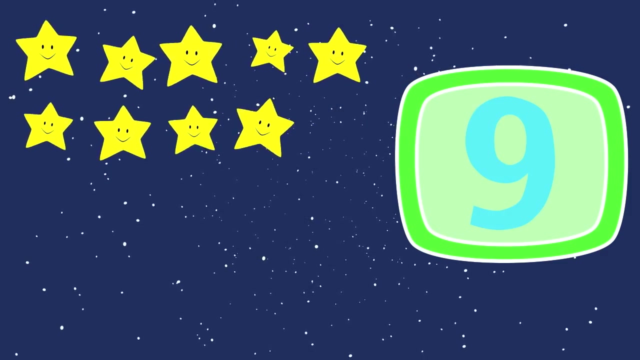 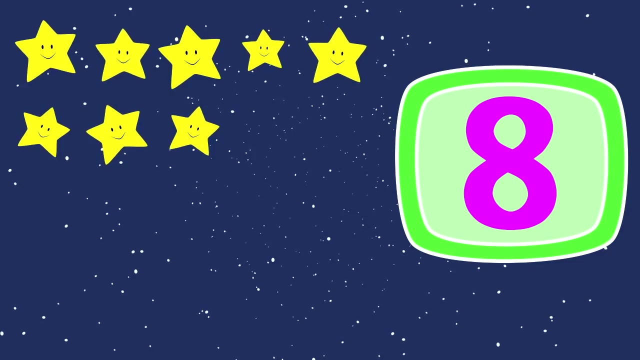 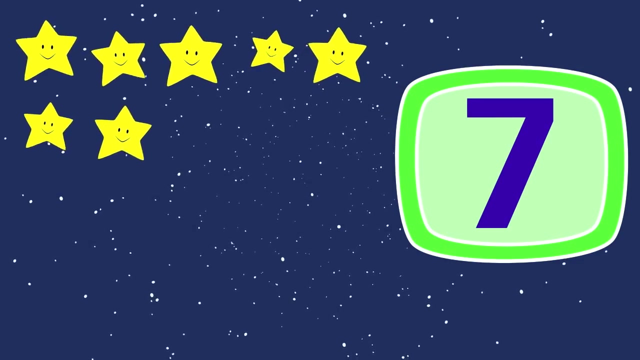 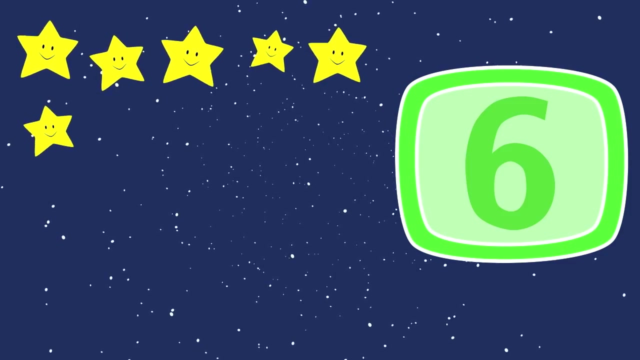 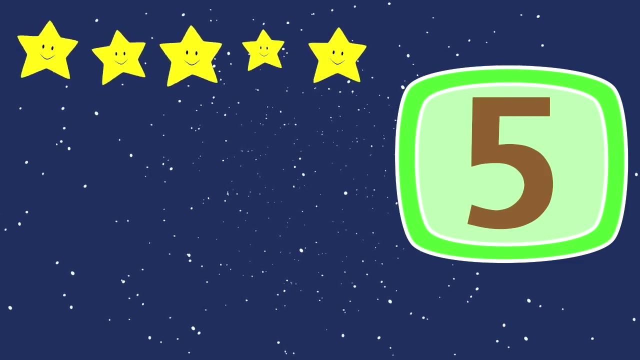 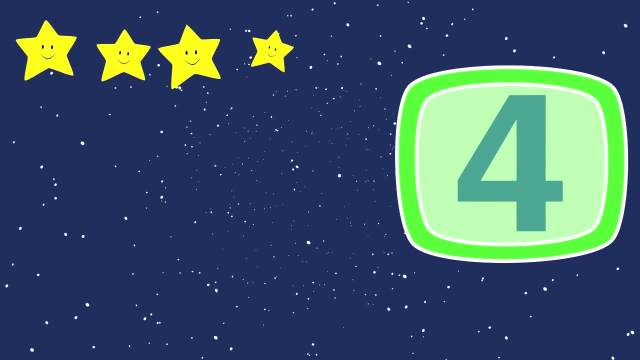 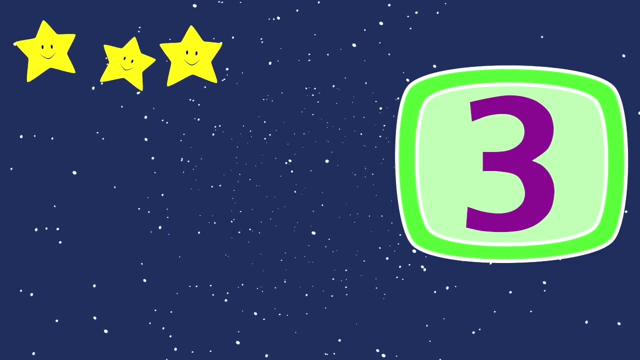 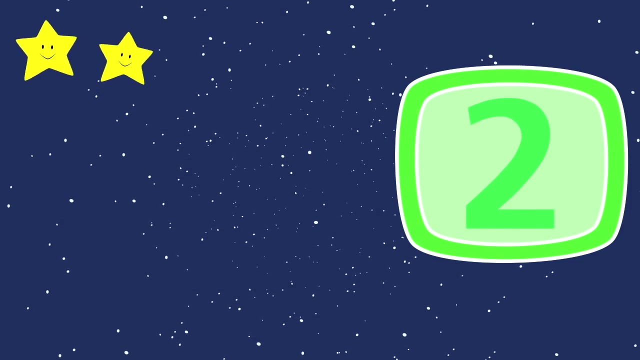 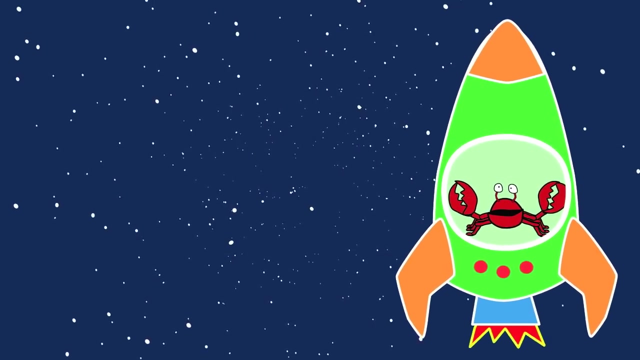 19,, 20, 22,, 24, 25, 25, 26, 27, 28, 29, 30, Thirteen, Twelve, Eleven, Ten, Nine, Eight, Seven, Six, Five, Five, Four, Three, Two, One. Fantastic. Now let's see how well you can count on your own. 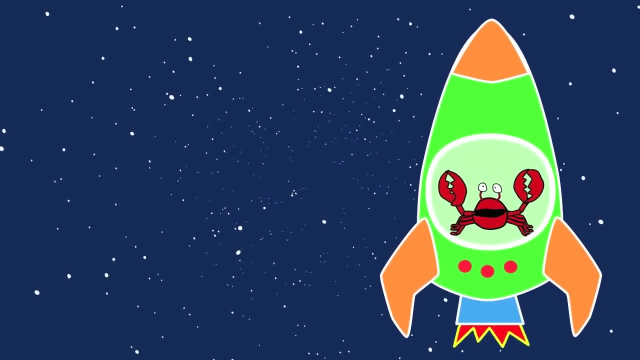 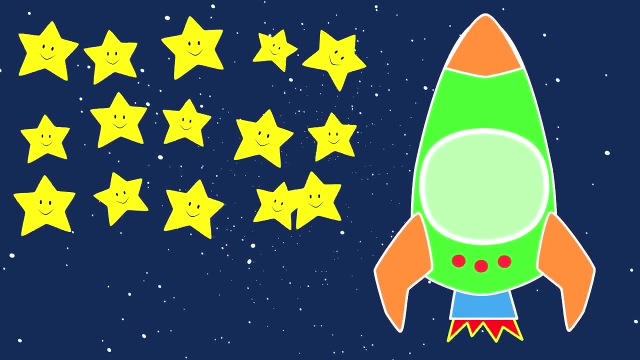 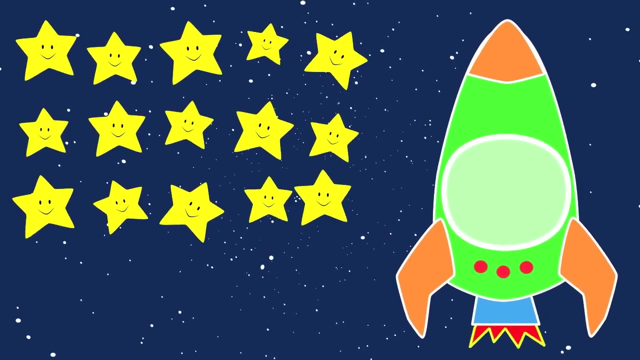 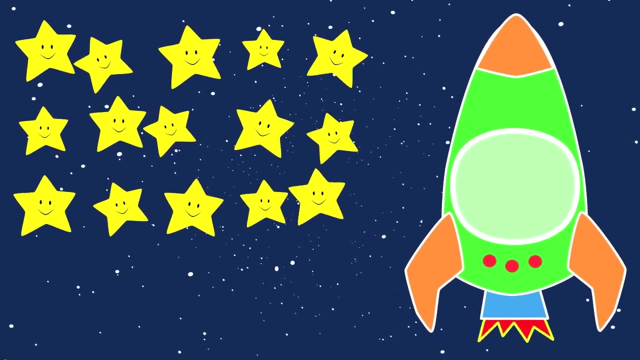 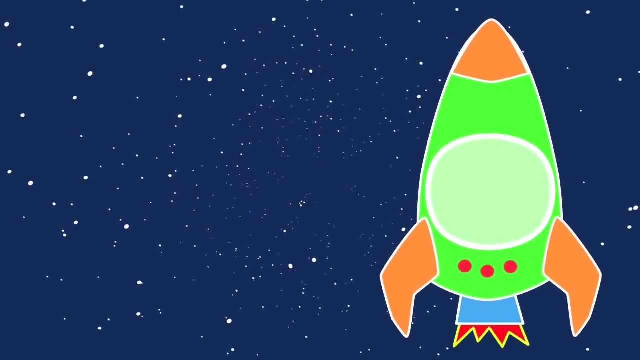 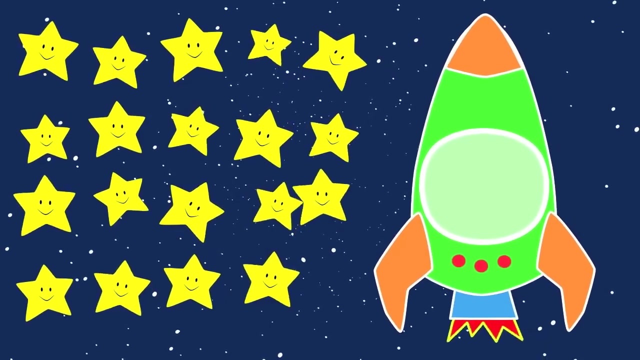 Count the stars in the sky and tell me how many. there are. One, Two, Three, Four, Five, Six, Seven, Eight, Nine, 10, 11, 12, 13, 14, 15, 16, 17, 18, 19, 20, 21, 22, 23. 24, 25, 26, 27, 28, 29, 30, 30, 31, 32, 33, 34, 35, 36, 37, 38, 39, 40, 41, 42, 43, 44, 45, 46, 47, 48. 49, 50, 51, 52, 53, 54, 55, 56, 57, 58, 69, 60, 61, 62, 63, 64, 65, 66, 67, 68, 69, 70, 71, 72, 73, 74. 75, 76, 76, 77, 78, 79, 80, 81, 82, 83, 83, 84, 85, 86, 86, 86, 87, 88, 89, 89, 90, 91, 92, 93, 93, 93.